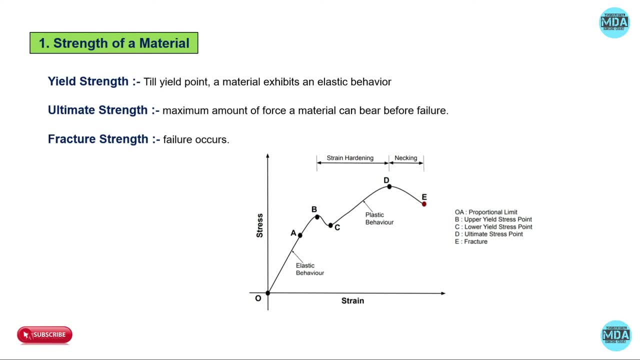 the ability of material to withstand the applied load without fracture, or you can say that resistance to the permanent deformation. As we know, when external load is applied on the material, some internal stresses are developed. The stresses causes the strain or deformation in the material. So at that time the strength of the material is very important during the product design. 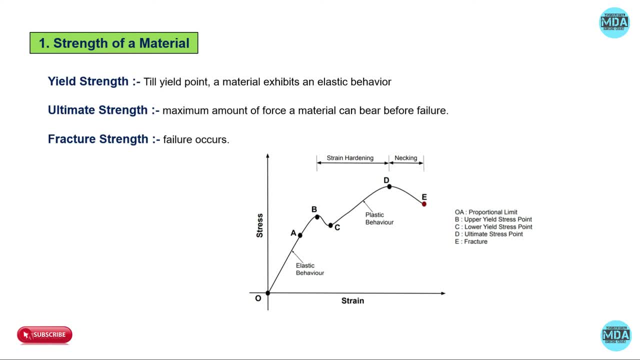 As you can see here in a stress-strain diagram, material is under elaboration of the material. So at that time the material is under elaboration of the material. So at that time the material is under elaboration of the material. So at this time we can define the. 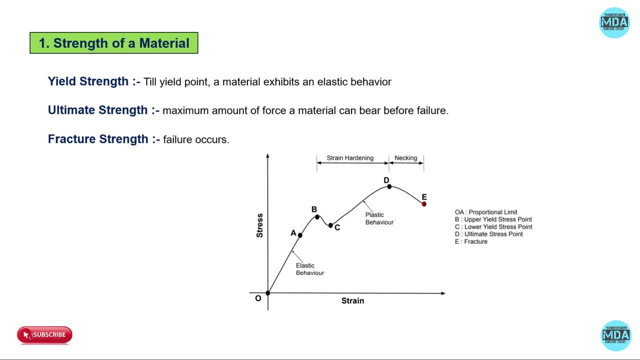 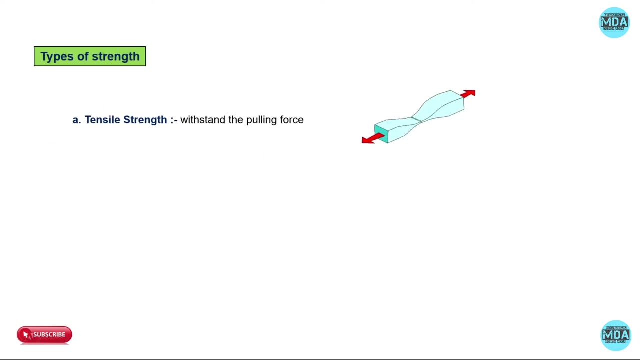 � мира is Route is occurs. As per the type of loading acting on the material, the different types of strength are tensile strength, compressive strength and torsional strength. Tensile strength, it resists the stretching or pulling. Compressive strength, it withstands the pushing force and the torsional 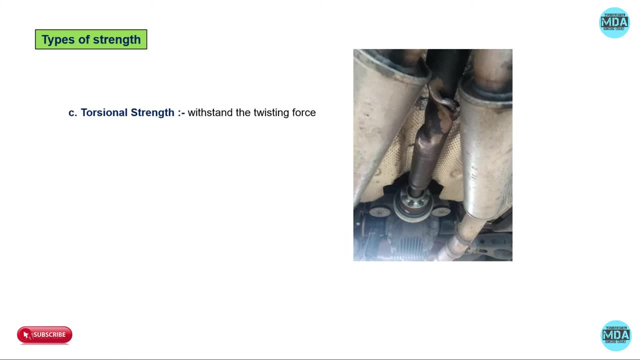 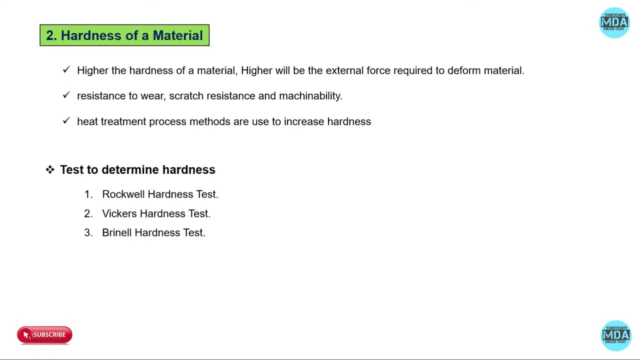 strength withstands the twisting force, like you can see in a propeller shaft. Next one, we have the hardness of material. So hardness- hardness you can define as it is a resistance to the scratch or cut- Hardness of material plays very important role in a wear resistance scratch. 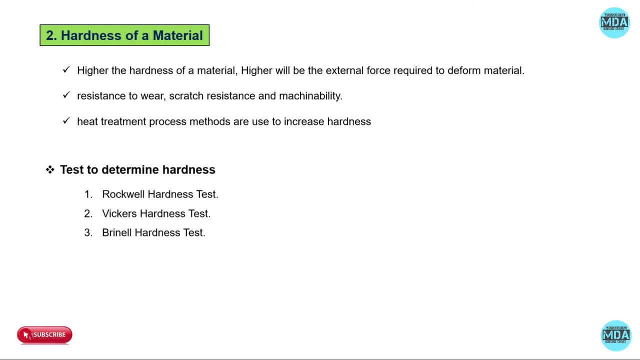 resistance and in a machinability. So the hardness can be increased by using heat treatment process. There are different types of heat treatment process So from that we can increase the hardness. So hardness of material is defined by number and determining the hardness we have different. 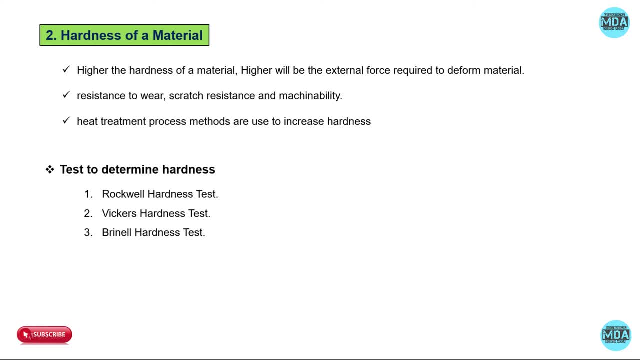 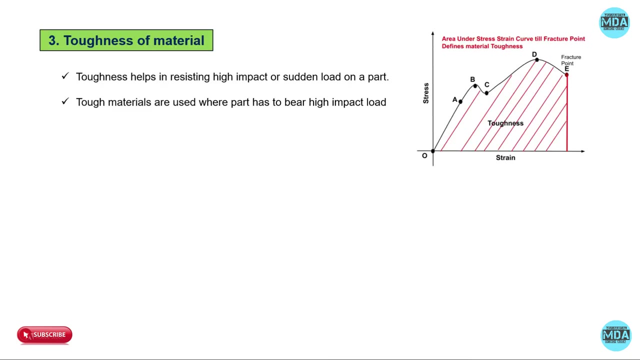 types of testing. So that is Brinell, Wicker and Rockwell hardness test. The diamond is a very hard material and it is used to cut the other hard material. Next one is the toughness of material. Toughness of material is very important when the material has to bear the 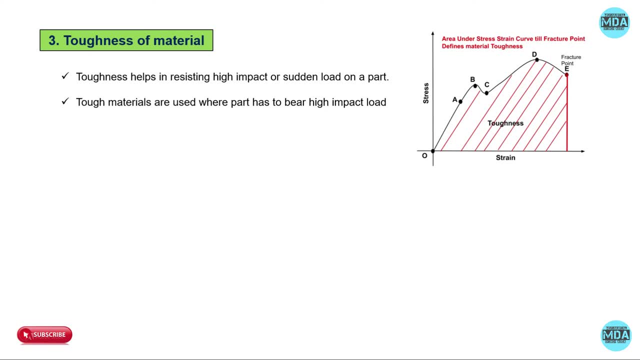 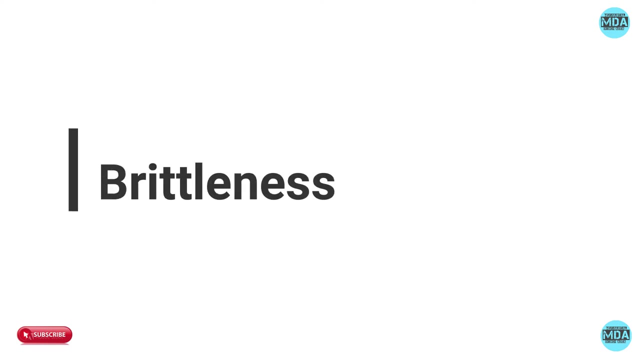 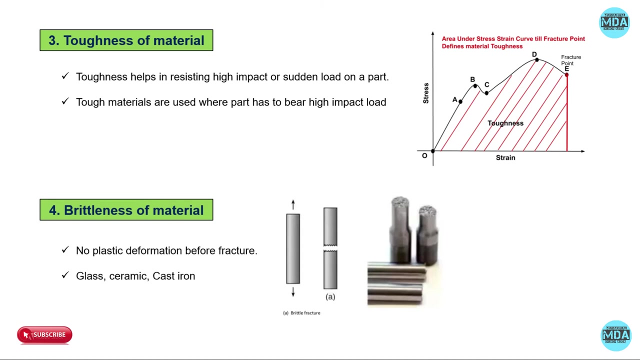 high impact or sudden load. It raises the high impact and sudden load on the part Mathematically up to material fracture point the energy absorbed per unit volume. that nothing but the toughness. as you can see in the stress-strain diagram, Brittleness is a contrast to the toughness. It is the tendency to show no strain or plastic deformation before the fracture. 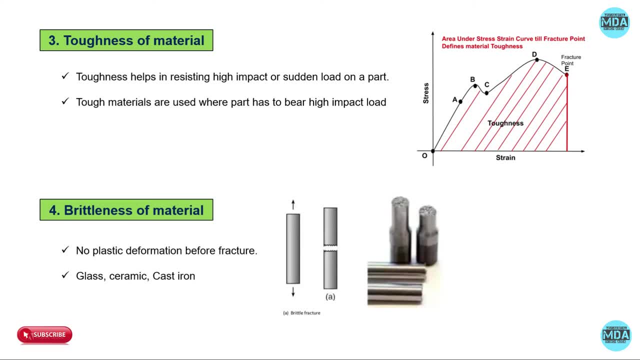 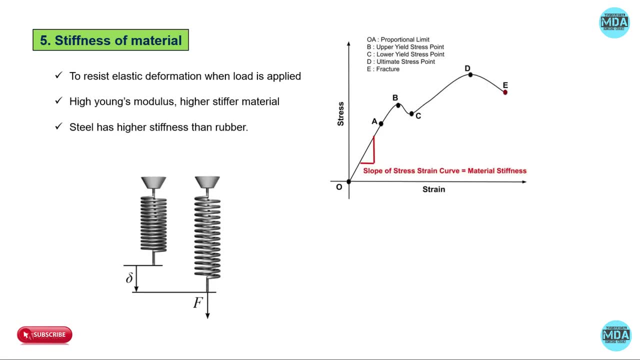 You can see the example of glasses, ceramic, cast iron. These are the brittle material. Next one is the stiffness. So stiffness is nothing but the property of material that raises the elastic deformation or deflection while loading. So it is the property of material. 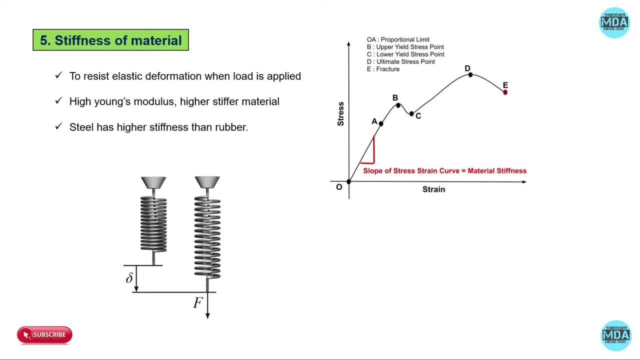 that raises the elastic deformation when the load is applied. So the stiffness of material is nothing but the slope we are getting from the stress-strain curve in the elastic limit. Steepness you can understand from the Young's modulus. so which is the ratio of stress to the strain? Higher the Young-Yeng's. 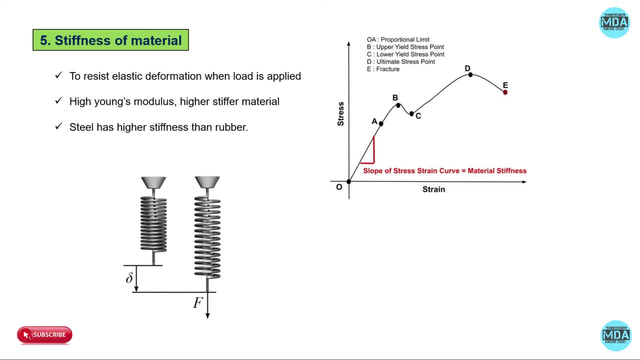 modulus and higher will be the stiffness of material. Stiffness is nothing but the rigidity. of the material Still has higher stiffness than the rubber When the material is subjected to various load conditions and audio not available. This is due to different Estoic methods which are used in gamma trabalhar test. The material is submitted, but the stability 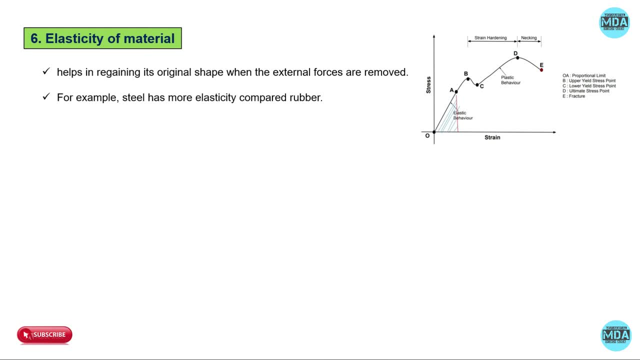 is not there, This means the resigned joint is inadequate. the joint is dependant on the regain its shape and size after removal of loading. so this one is a elasticity of material which which can regain its original shape and size after the removal of load area under the stress strain curve till the end point is known as: 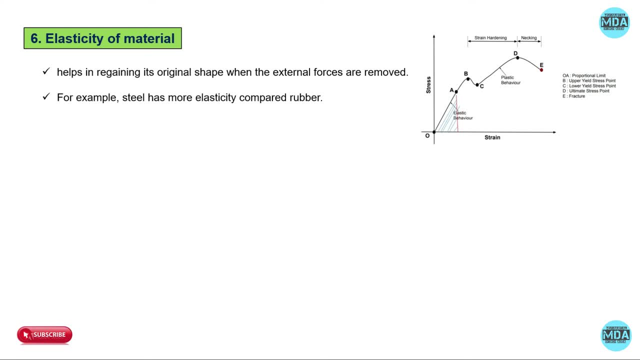 elastic behavior of that material. every material has some elasticity and it is major in terms of Young's modulus, which is the ratio of stress to the strain. next one: we have the plasticity of the material, when material is subjected to various load condition but does not regain its original shape and size after. 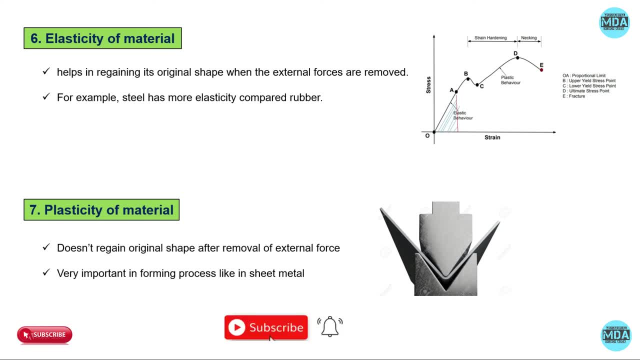 removal of load. it is the plasticity of that material. after the end point the material behaves as a plastic, so it doesn't regain its original shape. so the plasticity of material is very, very useful in the sheet metal operations, like in the forming operation. so next one, we have the ductility of material. it is the property of material. 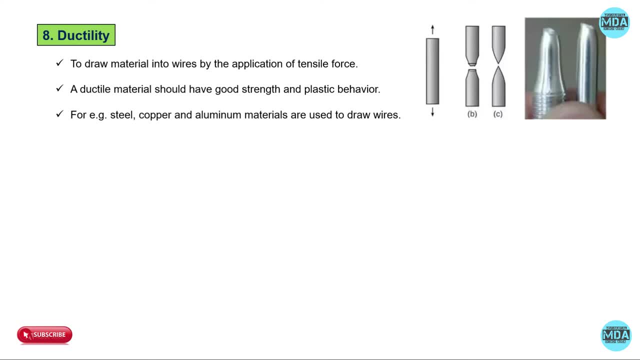 which can draw into a wire with the application of tensile force. so ductility should have the strength and the plastic behavior. so ductility- it is a permanent reduction in the cross-section area- can be achieved by pulling a rod through a die to produce a wire without breaking. if the temperature of material increases, the ductility is. 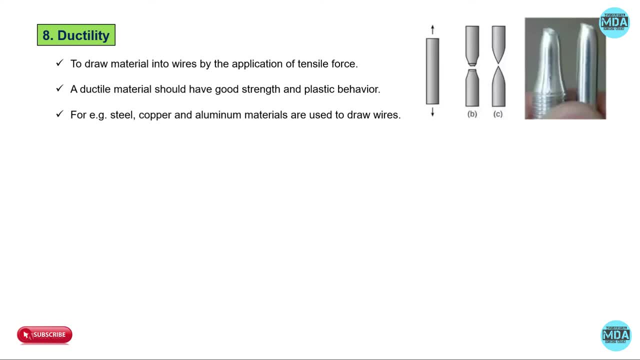 decreases. steel, copper, aluminium materials are used to draw wire. next we have the millability. the millability helps in converting the material into thin sheet. millability of the material can undergo permanent deformation in all direction under compression, by hammering, by pressing or by rolling, without cracking. 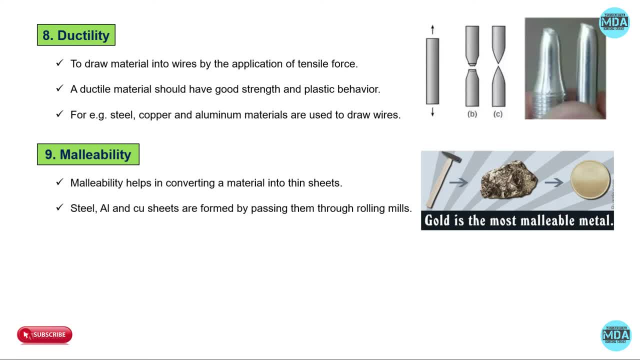 so without cracking it can undergoes permanent deformation. the applications are in forging, sheet metal, sheet manufacturing. so here the plasticity is essential. but millable material need not to be strong. millable increases with the temperature, as here you can see, gold is the most millable. 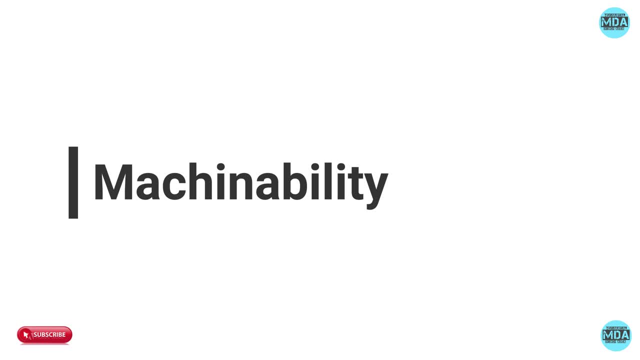 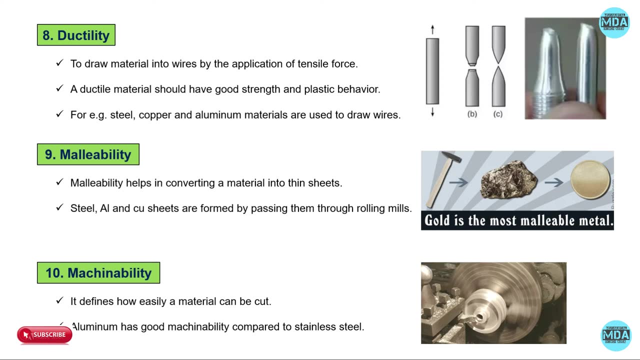 material. next one is the machinability. so machinability is the process of breaking objects. we can define as how we can easily cut the material or remove the material, like on a cnc machine, lathe machine and milling machine. the material must have the good machinability, while 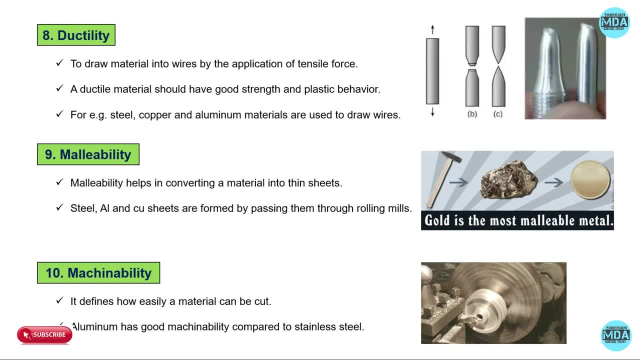 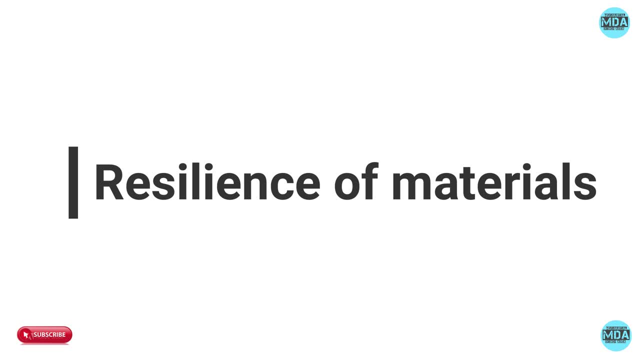 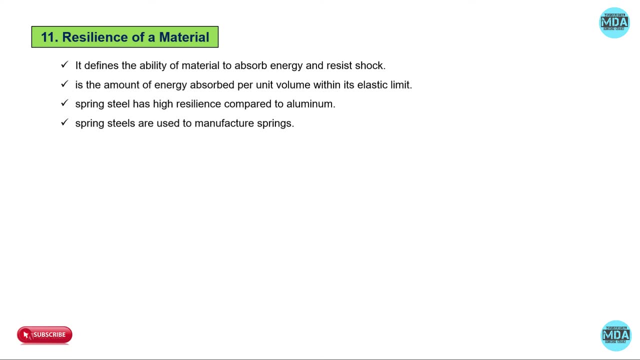 drilling while face cutting. so material must have good machinability so that we can easily remove the material. next one: we have the resilience of material. resilience is the property of material that defines the ability of material to absorb the energy and the shock loading. so the resilience is